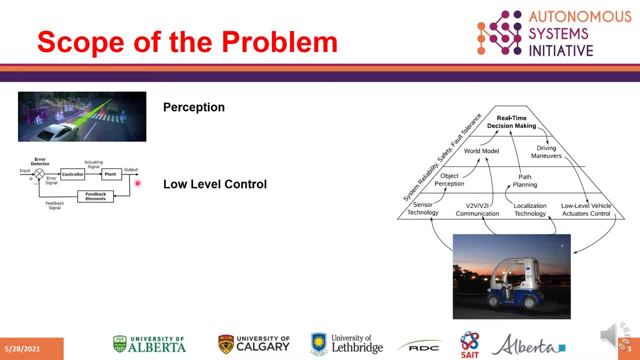 meta-actions are translated into low-level controls. For example, if we need to drive faster, how much fuel we're gonna need. And the next section is decision making, And this is what we are going to solve here. If we have already solved the perception problem, if we know about low-level controls, how optimally we're 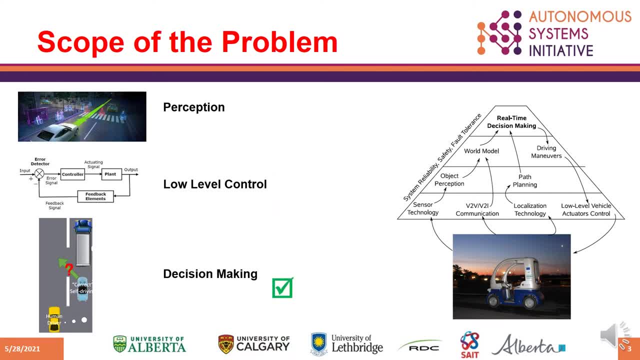 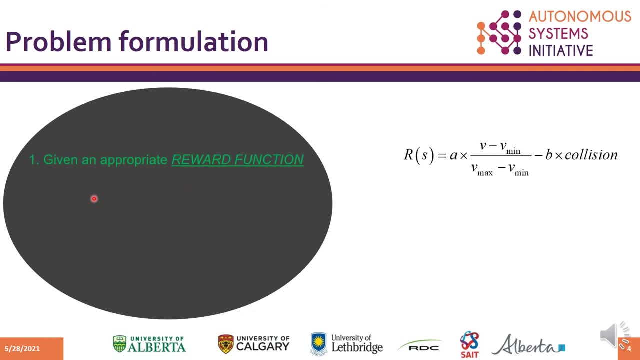 gonna make decisions. All right, let's formulate the problem before solving it. The first step is defining an appropriate reward function because, as I already said, we are gonna use the enforcement learning setting to solve the problem, So we do need an appropriate reward function. 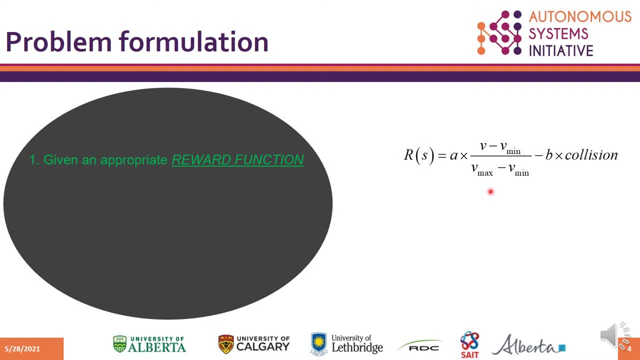 And the most usual case in autonomous navigation scenarios is to give high positive value to the cases that we are going, that we are driving quickly where A is an appropriate parameter, and huge negative value to the cases that we encounter collisions, which will be 1 when we 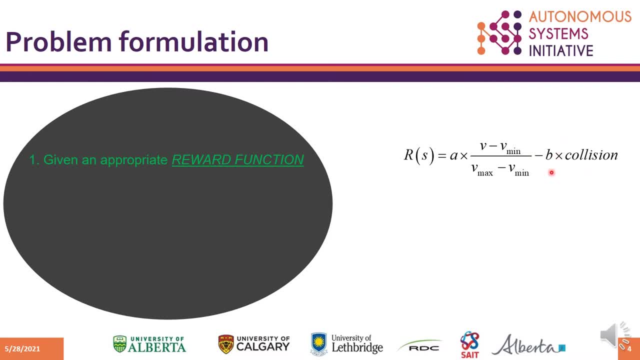 face the collisions, and B is also an appropriate parameter. Also, we assume that we have access to the traffic model, so we do know how many lanes are in the environment and we do know about the distance between the lanes, and we also assume that the number of lanes is constant in the problem. 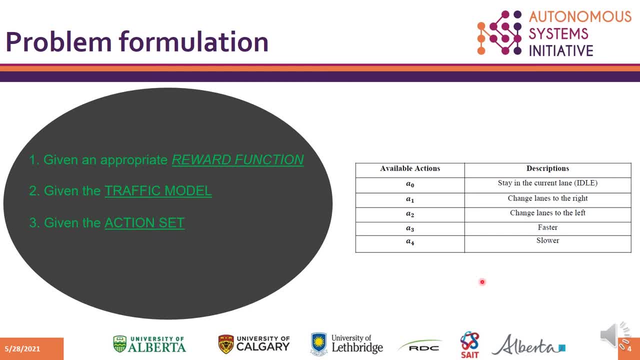 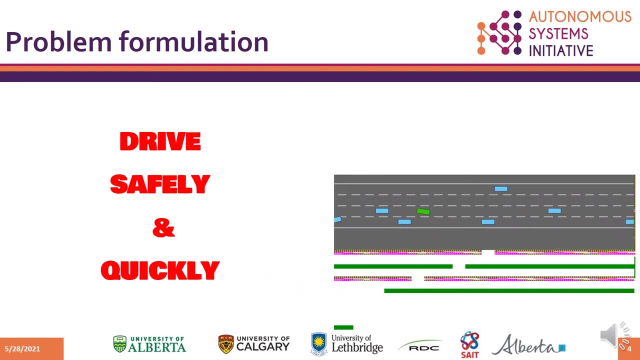 Also, we assume that we have access to the constant number of actions that we are going to select between each of them at each time step, And the problem is, given those assumptions, to drive as quickly as possible without ever having a collision. Let's see what's the novelty here. 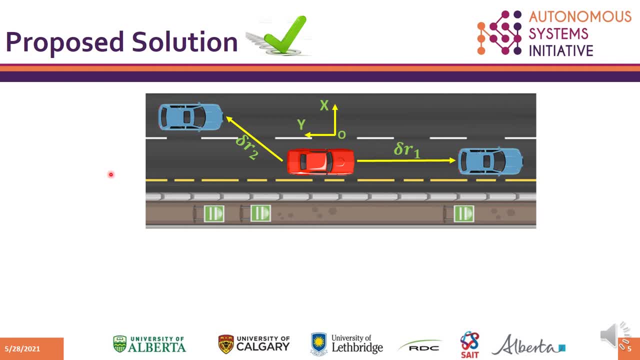 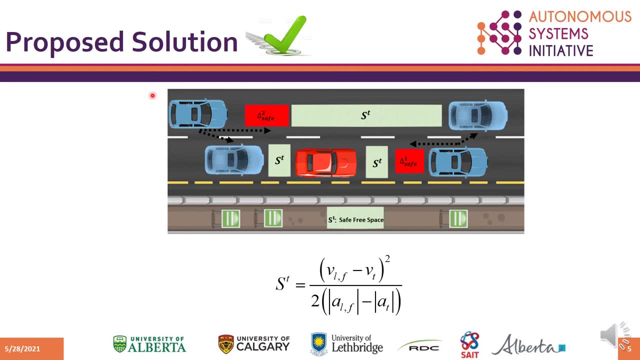 Consider a simple scenario of autonomous navigation. Okay, it's obvious that the optimal decision-maker will never, ever make unsafe decisions, so we can always be careful. We can also use basic rules from physics to form the safe distance to the adjacent vehicles in the environment.